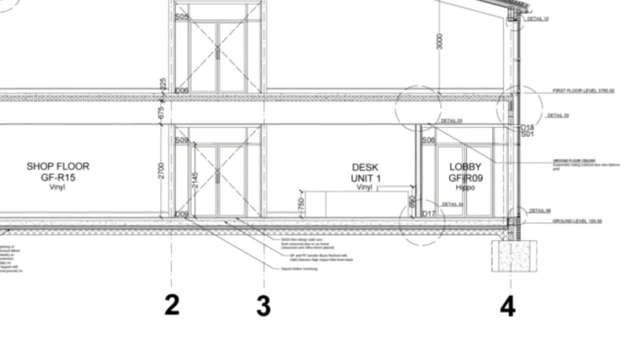 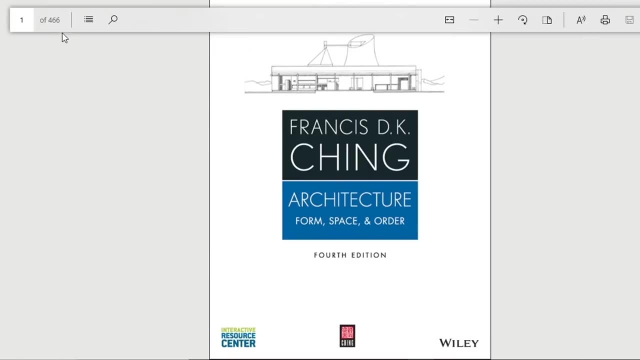 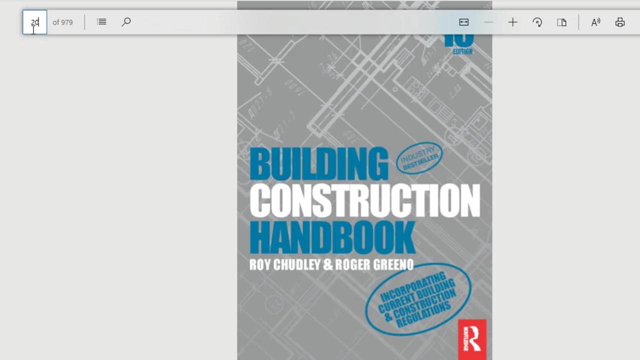 calculus or physics. Truth is, I was so proud of myself for finishing this, But in the end I did finish it, and you will too. You just need to do research and learn from other drawings and basically copy. Yes, it is not plagiarism if you draw it yourself or you can say courtesy of and 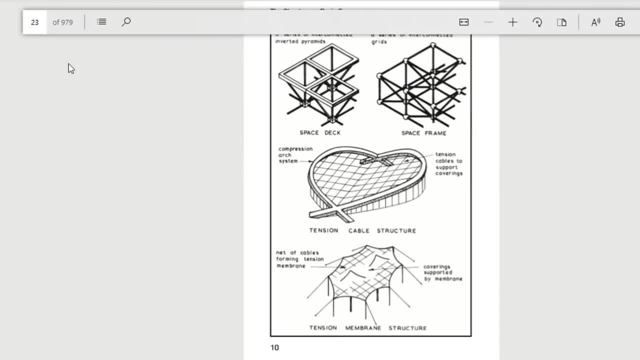 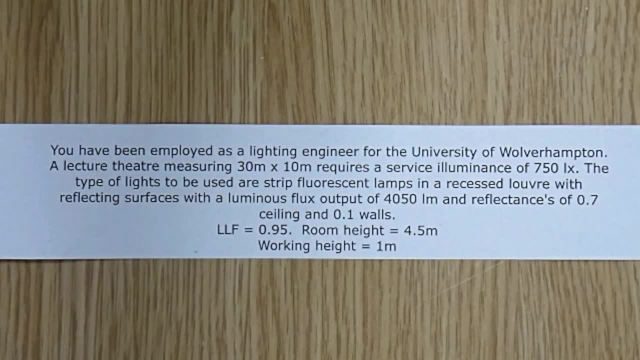 then the manufacturer's name, And I mean the construction drawings only Don't plagiarize designs. You also need to be able to solve simple equations where you substitute values for variables and solve for x. You also need to be able to solve simple equations where you substitute 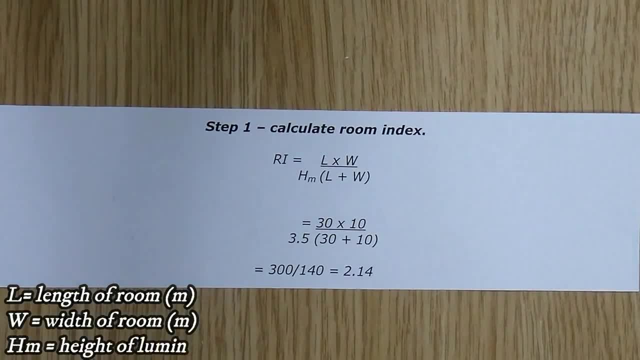 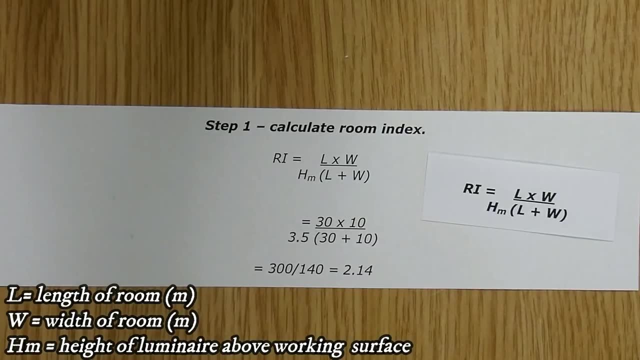 values for x and y. Those equations all have steps and if you follow them well, you're good to go. I've made a video about how to calculate how many light fixtures you would need for space and I will have that linked in the card for you to check out to get an idea of one of the formulas that I used. 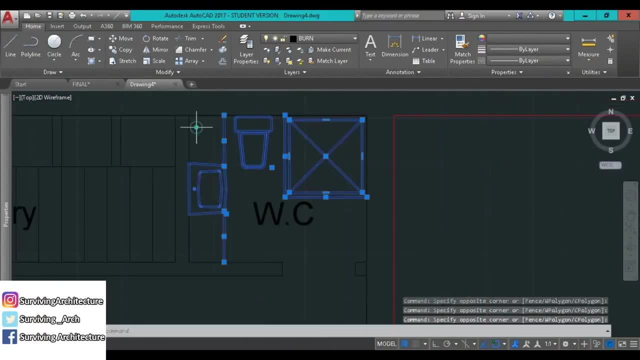 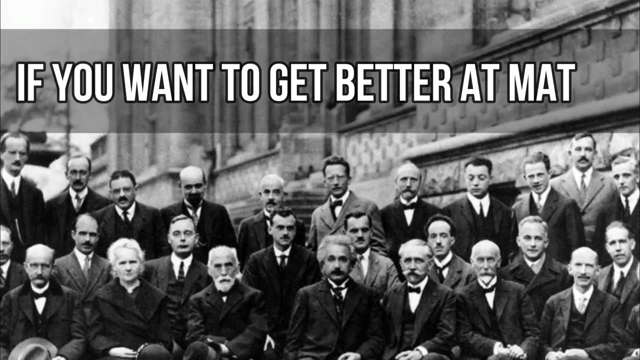 I've also studied at another university where we had more physics than the one I am currently studying at, so it depends on the university as well. If you want to get better at math, do a lot of math. Find someone who is good at math and good at. 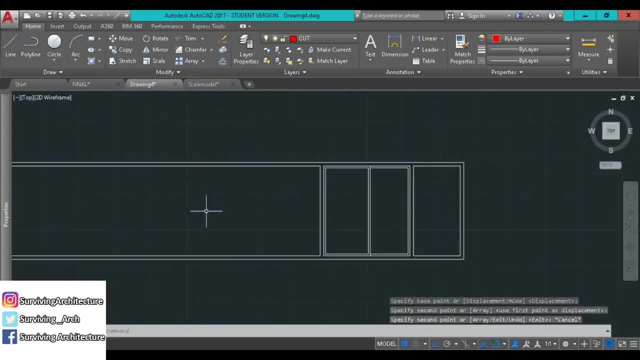 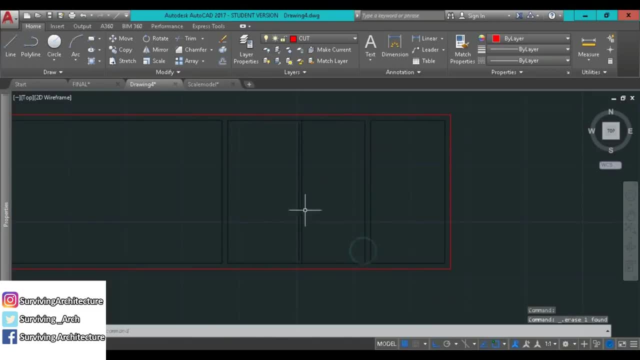 teaching. You also need to note that most of the architectural work now is leaning towards digital-aided design, meaning software that will help you design your building and your structure. So if you're not sure about how to calculate something or the length of an arc, a volume of 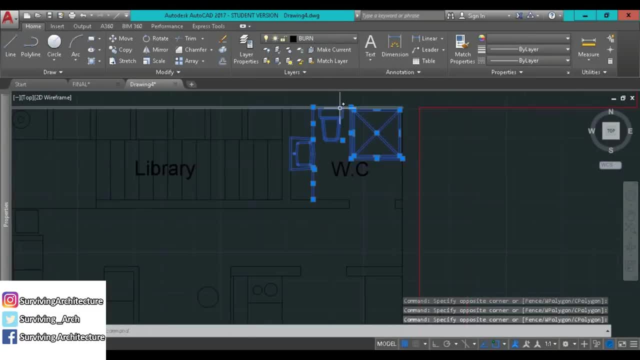 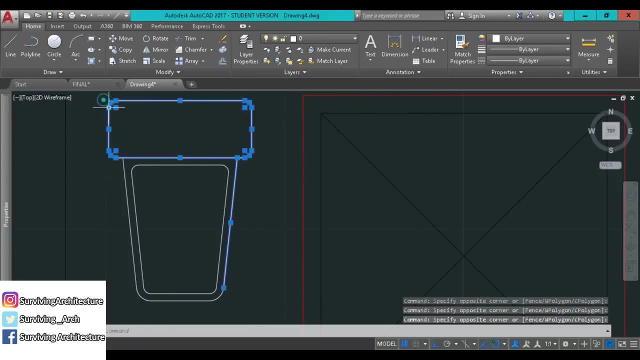 space, that all can be measured in CAD and other softwares. In conclusion, I think you should understand the principles and concepts of math and basic physics, but you don't have to be the next Albert Einstein, and we all have calculators and you don't need to memorize the 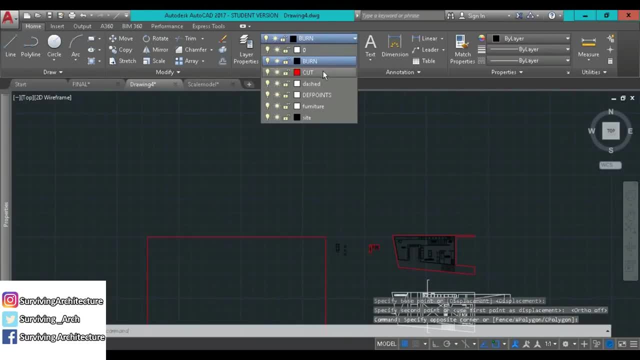 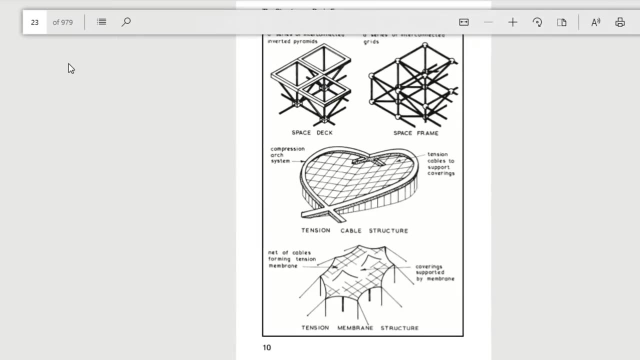 diagrams, formulas- as these will all come with experience being on site- and reference materials, because that's what reference materials are for. So don't be discouraged if you're not strong in math. It's a skill like yoga or riding a bicycle: You can learn it, and it should not be a source of 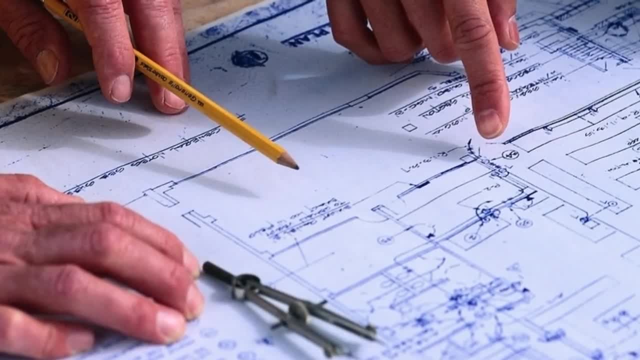 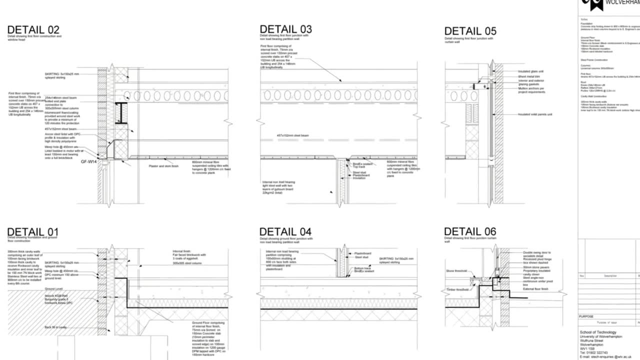 stress And don't forget when you're out in the real world, you won't be working on a project alone. You can get into a big firm where the engineering department handles all the structural calculations and you just do the details or the research. You don't need to have a lot of time to